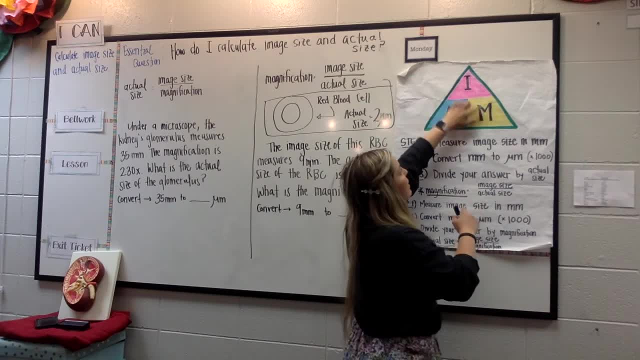 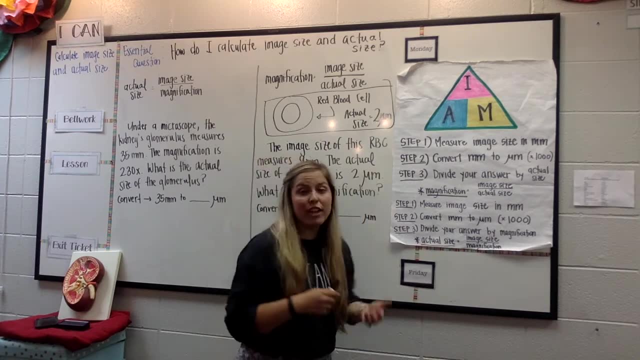 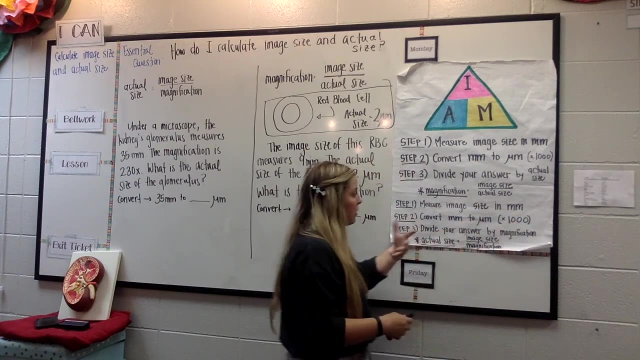 for image size divided by actual size. So M equals I over A, Magnification equals image size over actual size. Now, if we were looking for actual size, which will be fairly common, we will measure the image size or they will give us the image size in a millimeter size. We must convert millimeters to. 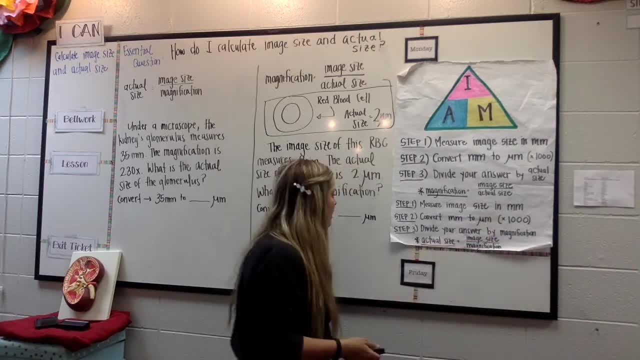 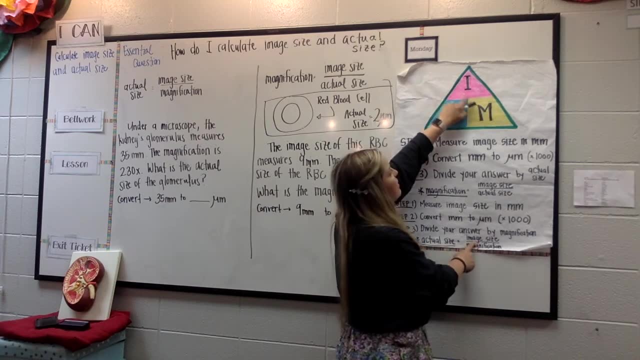 micrometers, And to do this we just simply multiply times 1000. And then we will solve for actual size. So, if we're using our triangle, actual size equals image size divided by magnification. So that's just a simple way to use this formula to be able to understand these. 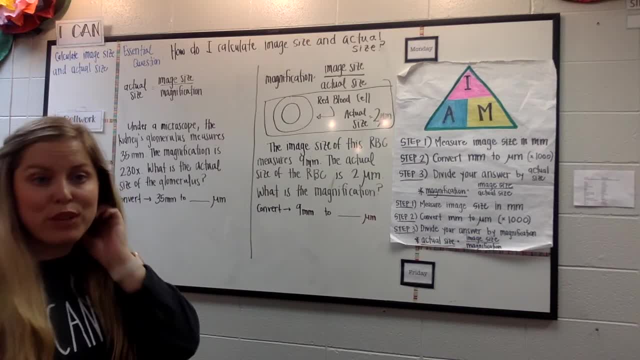 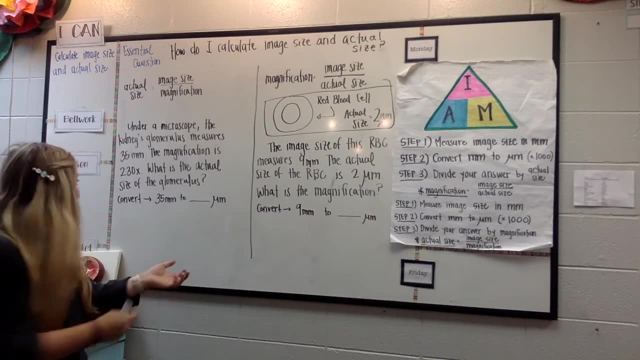 problems. Now. I have two problems drawn here on the board of examples of questions that you might see at the end of the year. The first question deals with a portion of the kidney as we see it under a microscope. So I have a depiction of a kidney here And we're talking about this question, the glomerulus. It's one of the little filtering units, how our kidneys filter out the good and the bad in our body. So for this question, under a microscope the kidney's glomerulus measures 35 millimeters. The magnification is 230.. What is the actual size of the glomerulus inside of your 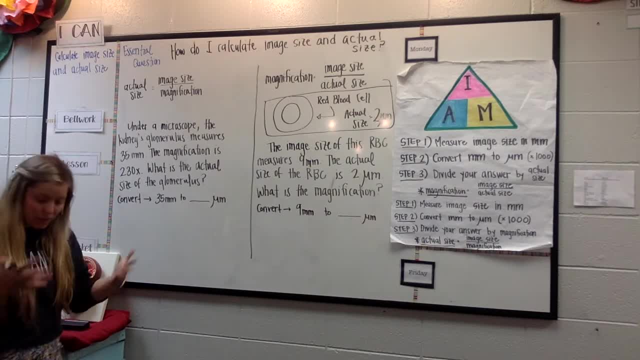 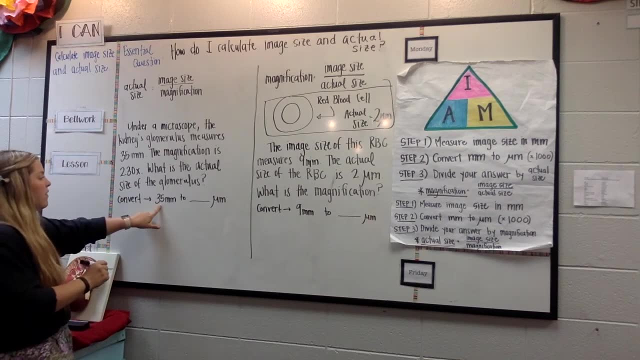 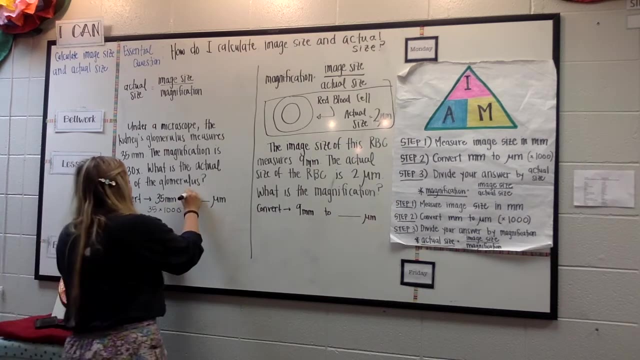 body, So we know what it measures from the image that we're looking at And what is the actual size of the glomerulus. So the first thing we're going to do is convert 35 millimeters to micrometers, And to do this, we just simply say 35 times 1000.. Okay, so that gives us 35,000 micrometers And the 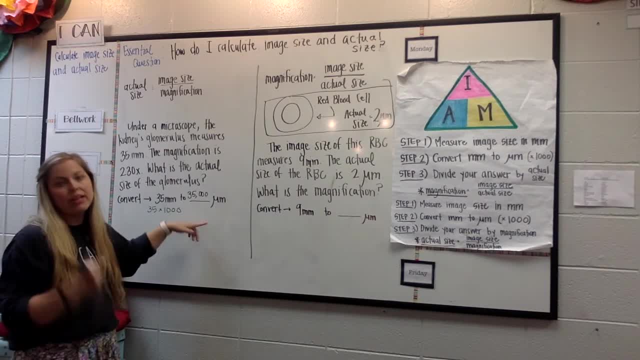 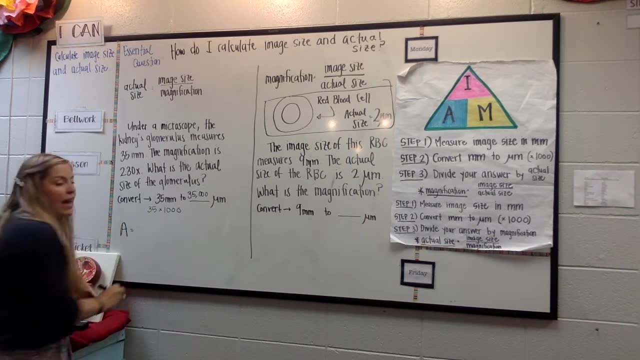 micrometer is always going to look like this M with a little tail on it. That's how you can decipher between a millimeter and a micrometer. Now let's solve for our actual size, And I'm just going to use an A A for actual size. That's going to be image size over magnification. 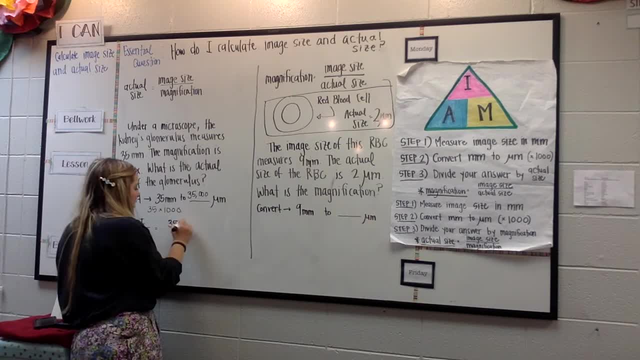 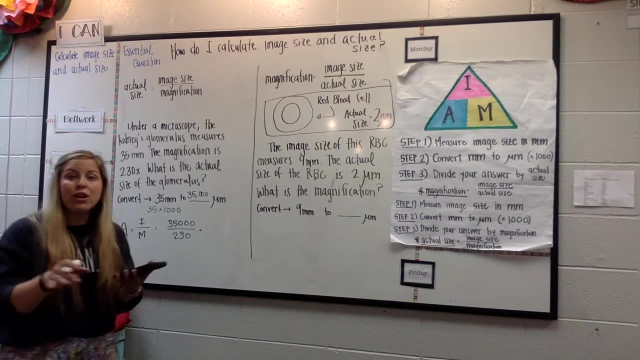 So if we have our image size, which we converted to micrometers, we have 35,000, divided by our magnification, And that was 230.. Okay, Now, if you have a calculator, this is where you would get out have to do some calculations, If you're. 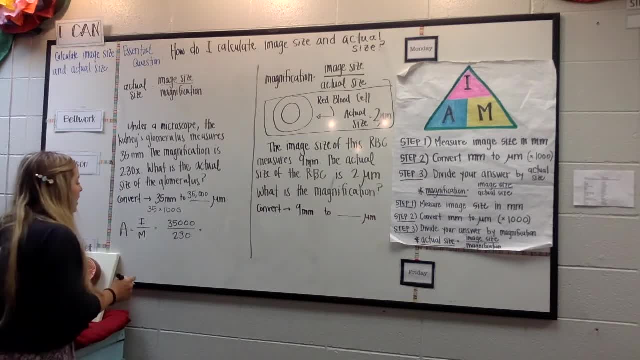 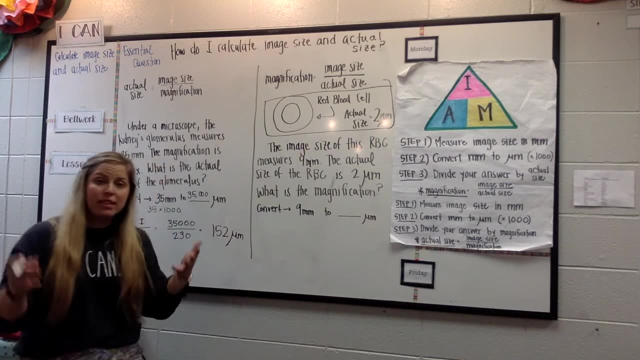 working at home. your cell phone should have a calculator on that. I've already done my calculation And that's going to be 152 micrometers. Now if, for some reason, your question asks you to transfer that back to a millimeter, you would just divide by 1000. So that would give you 0.52 millimeters or that size of a glomerulus in millimeter form, But for us we can say 152.. 152 micrometers is the size of your one glomerulus inside the Bowman's capsule of your kidney. 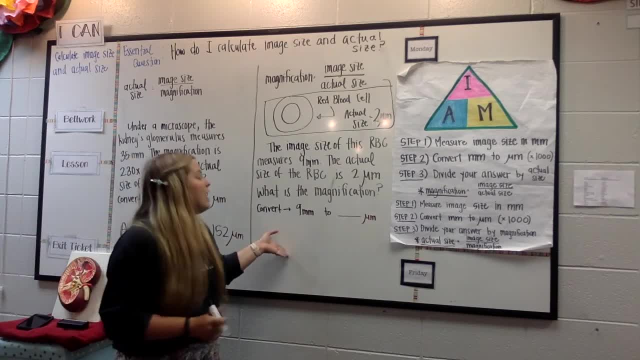 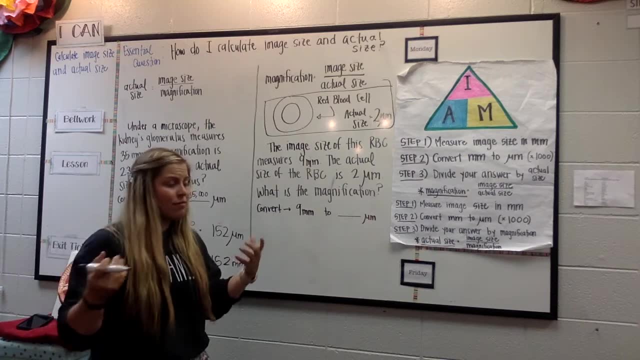 Pretty cool. Okay, Now we'll move on to another type of question that you may see where we're solving here for the magnification. So if you get a question about this, this is some sort of very, very small entity. for this It's the red blood cell, And we want to know how many times 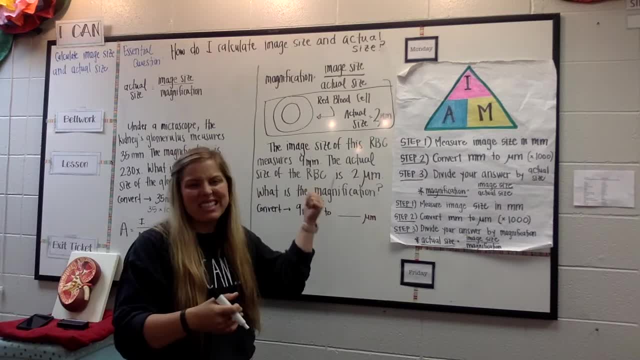 is this question or this image that you're seeing, because you would see this on an image with a picture, either in a textbook or a picture that you're seeing right now, and you would see this on a sticker, on a question. We want to know how many times did this microscope? 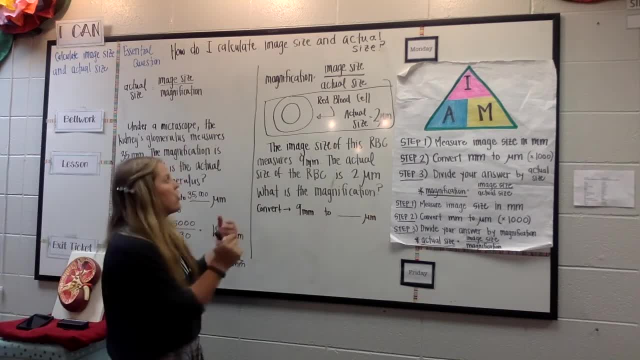 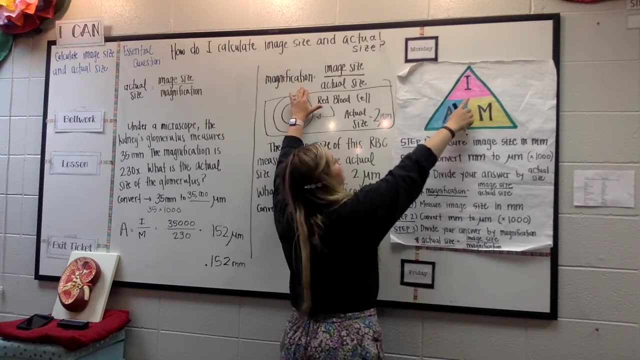 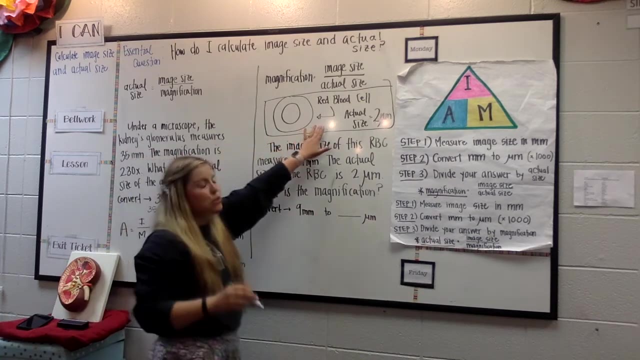 have to magnify this for me to see what it looks like and see its features. So for a magnification question, your magnification. so m equals i over a. so magnification equals image size over actual size. Now the red blood cell's actual size inside of your body, inside of my body, on average is two. 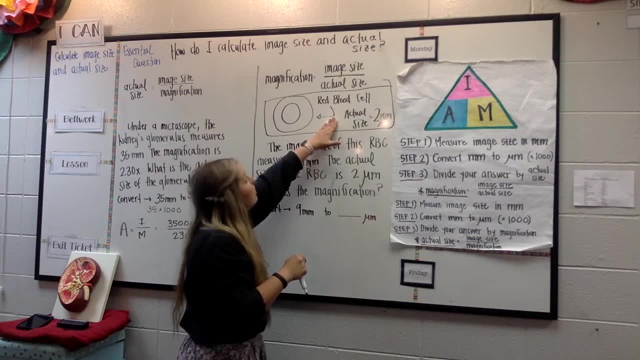 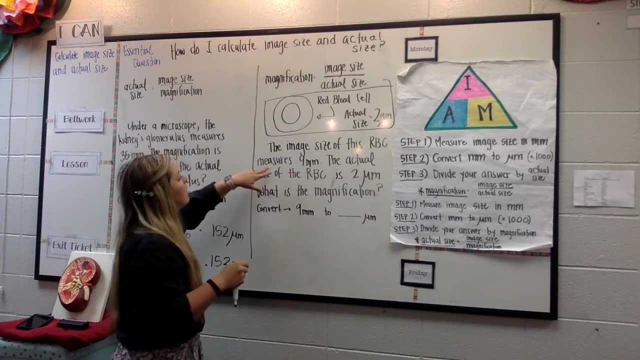 micrometers. wide cell is two micrometers, So the image size of this- and I put RBC on the board- red blood cell measures nine millimeters, So the picture that you're seeing. so pretend this is the picture. 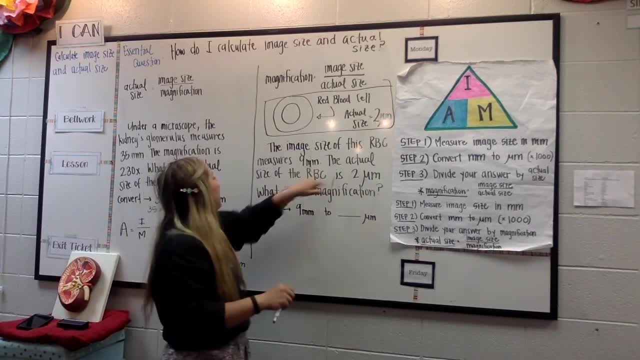 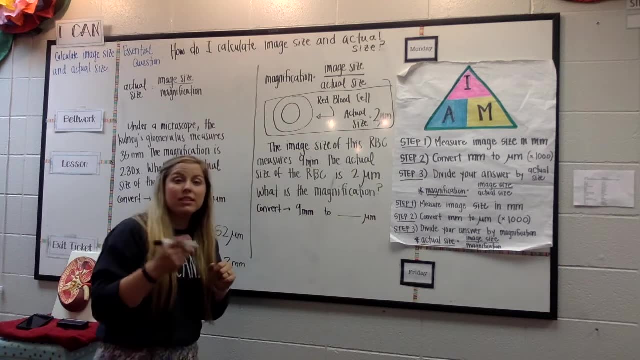 and that's not right in front of you, but it's just how the video is going to work. The actual size of the red blood cell, of course, is two micrometers. What is the magnification? Now, the first thing we need to do is convert your nine millimeter image into micrometers, So remember. 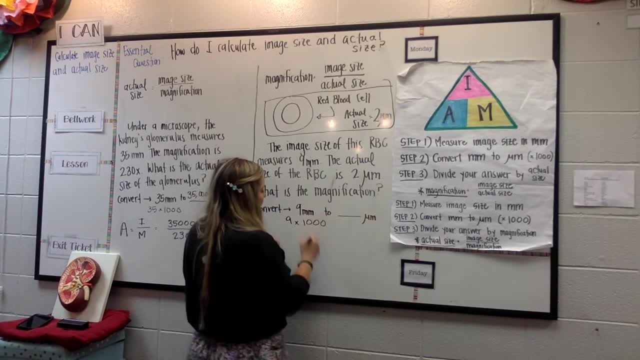 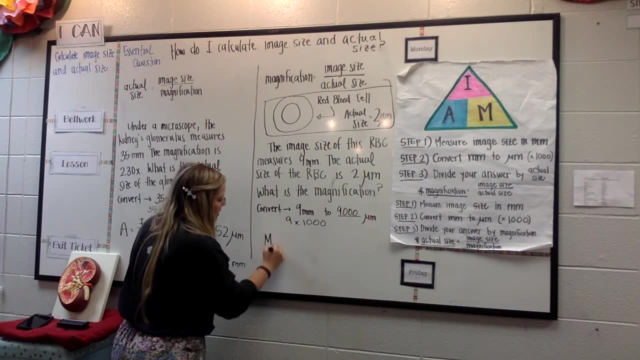 we simply multiply nine times 1,000, okay, which gives us 9,000.. All right, now we are simply solving for magnification. I'm just going to say M equals. So magnification from our triangle is image size over actual size. So M equals I over A. Now my image size, which we have converted to. 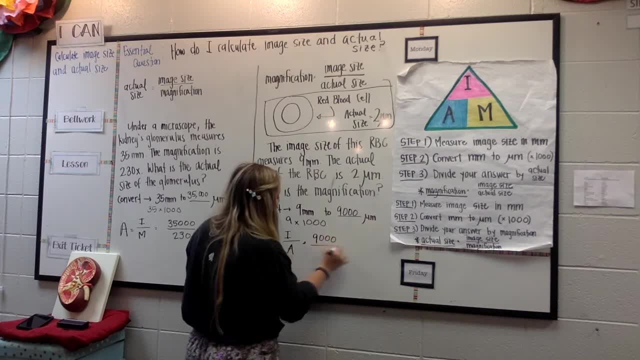 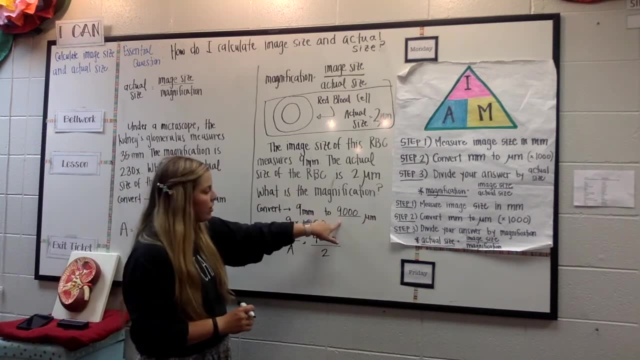 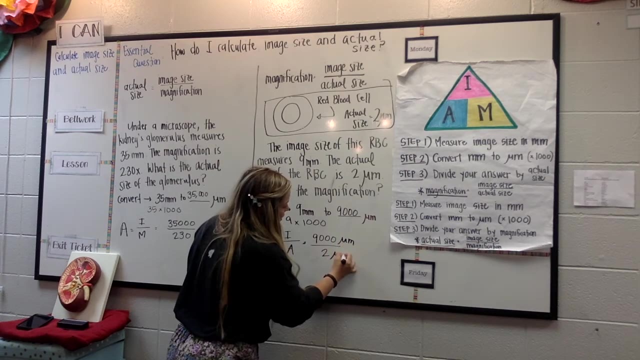 micrometers is 9,000 over the actual size 2,. okay, because we get the 9,000 from our conversion and then two micrometers, So if we wanted to put the units out beside it, we could. Okay. so our magnification: 9,000 divided by two.